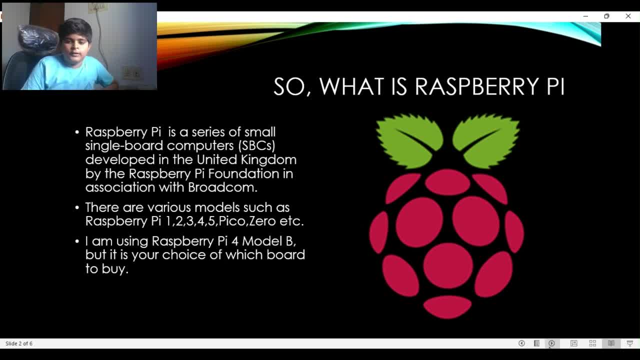 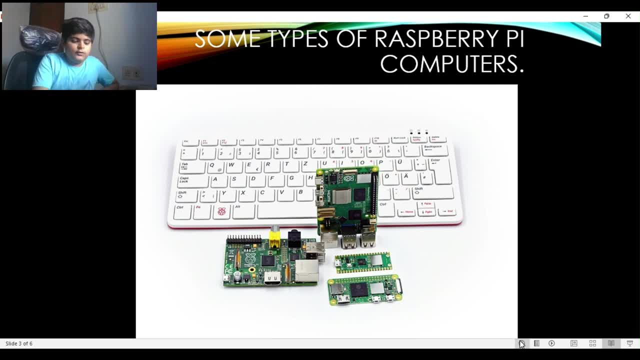 can even buy the previous boards. The process of installing Raspberry operating system: Yes, you can install an operating system inside the board. These are some types of Raspberry computers where you can install a Raspberry Pi 4 model. You can install a Raspberry Pi 5 model, You can. 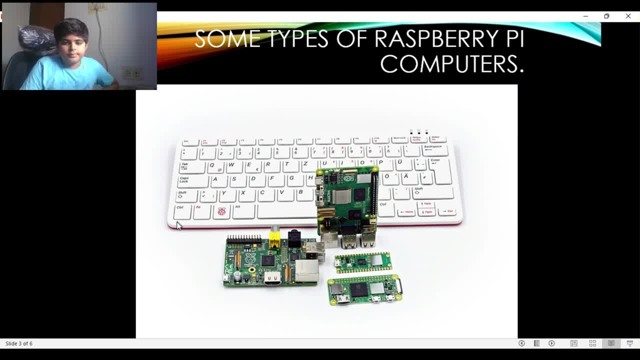 install a Raspberry Pi 4 or Raspberry Pi 4 held byあり Raspberry Pi 4 to turn off all these boards. You can do it any way. as buq transformed into a screen, There is no problem. But what is this keyboard doing here? Take a normal pc, put it into a desktop computer with. 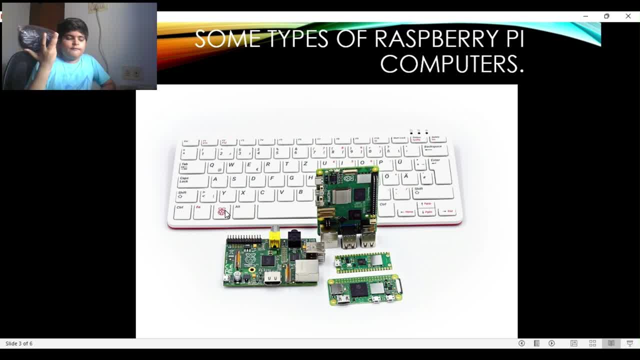 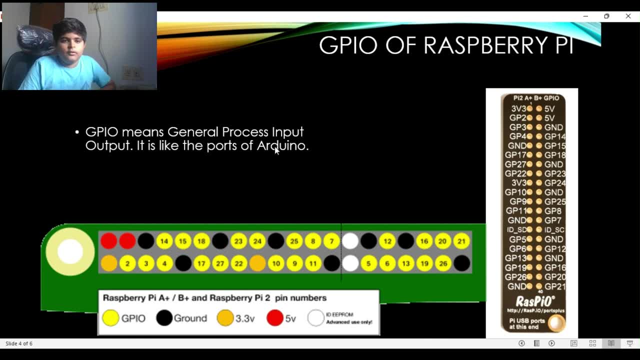 the help of my Hdmi cable. Hey, The processor is working, Plays us from the tablet to the laptop. This is the general process: input, output or GPIO. It is like the ports of the computer, It is like the audio video editing light, etc. 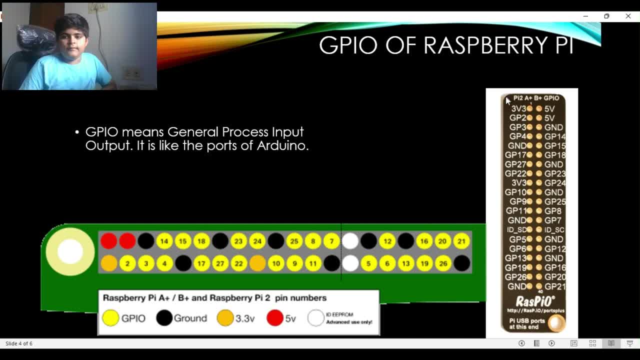 It is like the ports of a TV that Around 일 täll till Todaym long as Anyone can use it- of arduino. well, this is the reference pcb. you can put it on your board. in case you want, you can put it on your board. this is: this is another reference. you can find both of these on the. 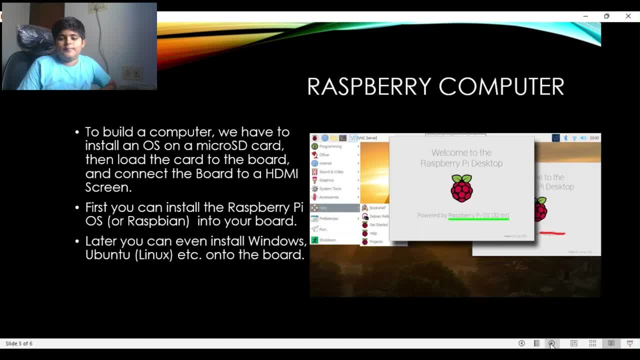 arduino web. i mean, sorry, raspberry pi website. this is the raspberry computer. to build a computer we have to install an os on a micro sd card, then load the card into the board and connect the board to hdmi screen. it seems like a large process, but i will show you how to do that. first you 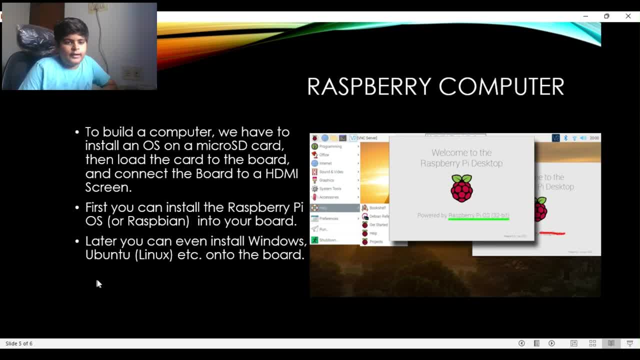 install the raspberry pi, os or raspbian onto your board, then you later you can even install windows. yes, you can build a personal computer of your own, but you need a better ram on your computer or ubuntu- i mean not computer board- and you can even use ubuntu or linux onto this board. 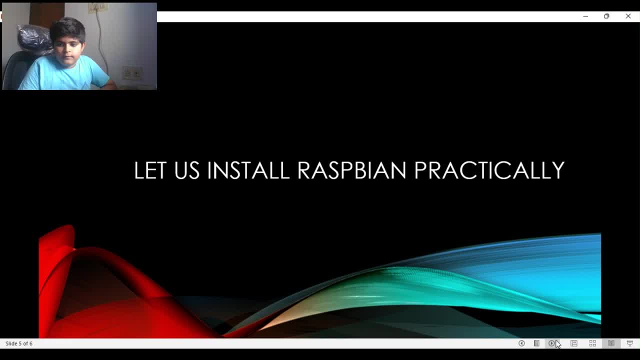 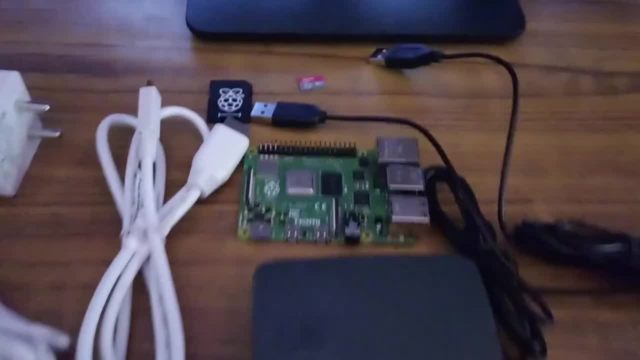 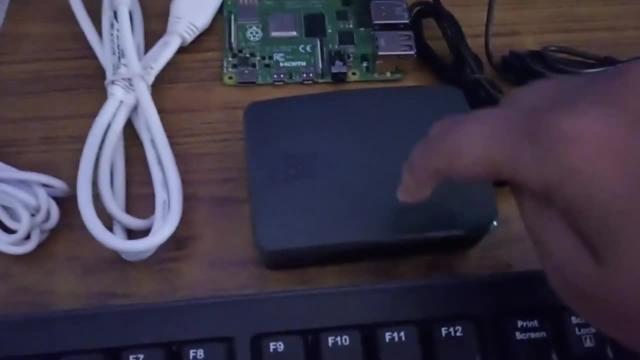 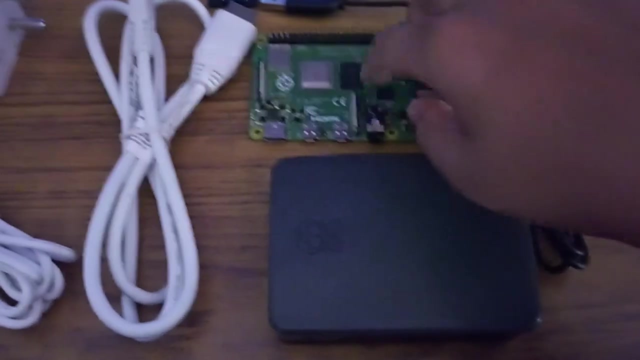 let us install raspbian practically first, we will learn what all things we need. this is the raspberry pi board. raspberry pi 4 model b of 4 gb ram. this is the official case of raspberry pi 4b. it is optional, but you can use it for not allowing dust to settle on the board. 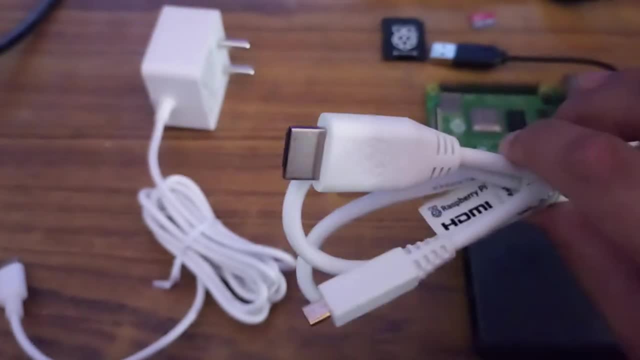 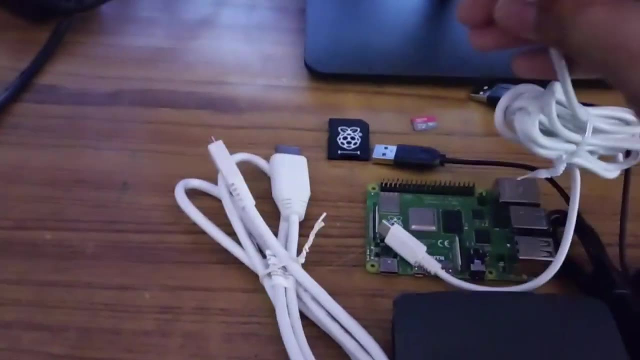 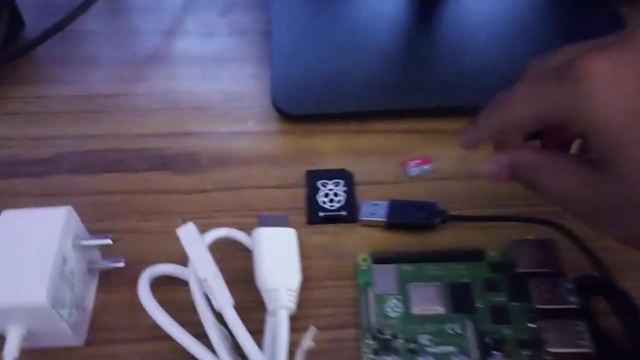 here is a micro hdmi to normalize the board and here is a micro hdmi to normalize the board- hdmi cable. this is the official adapter of of our power supply of raspberry pi. however, you can still use a normal fast charging mobile charger. here we need a small micro sd card, preferably 64. 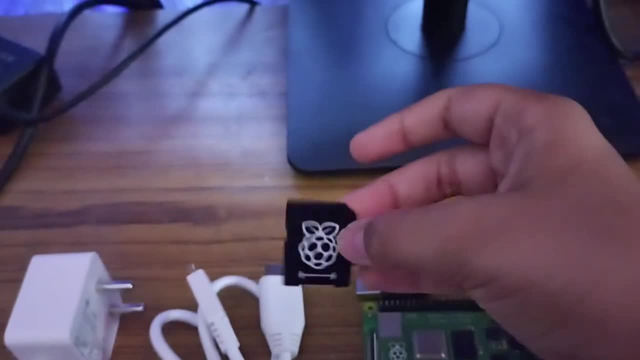 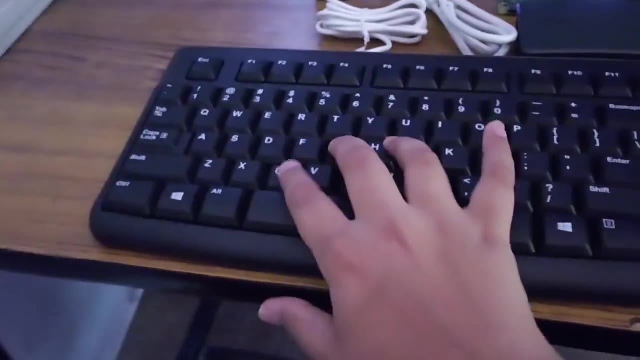 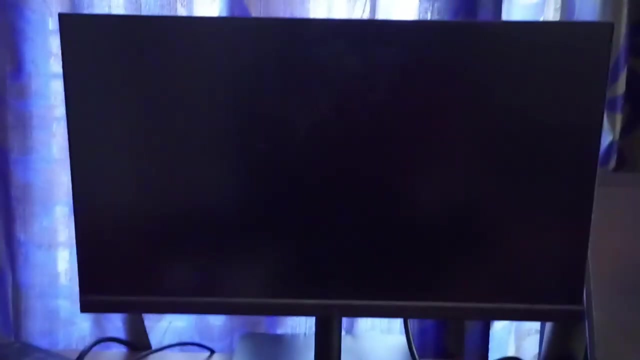 gb and this is the adapter which helps us to connect it to our laptops. and the most important thing we need is a wired keyboard and a wired mouse. both of them are important, and there is requirement of a hdmi screen. if you don't have a monitor like this, then you can use a normal tv. 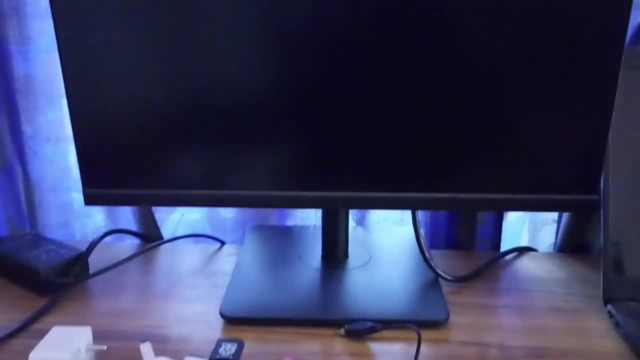 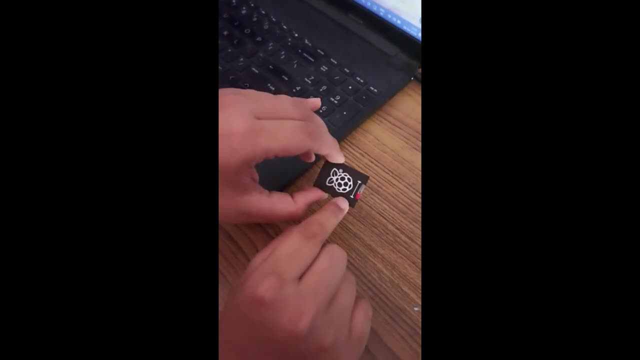 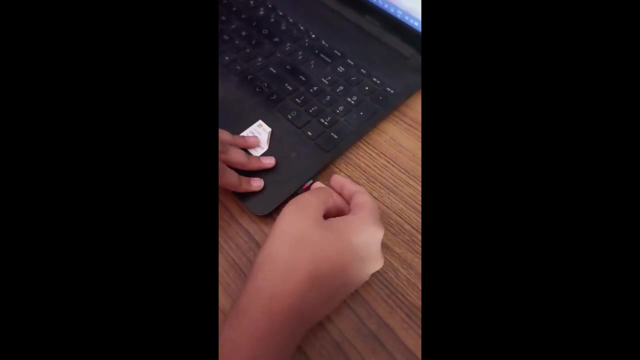 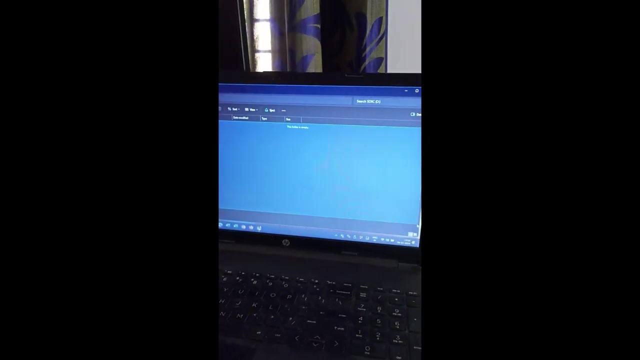 which has hdmi connections. as you can see, i have inserted the micro sd card inside the raspberry pi micro sd card to normal sd card adapter. i'm going to insert it inside the of the computer which will show me this folder. as you can see, this SD card is 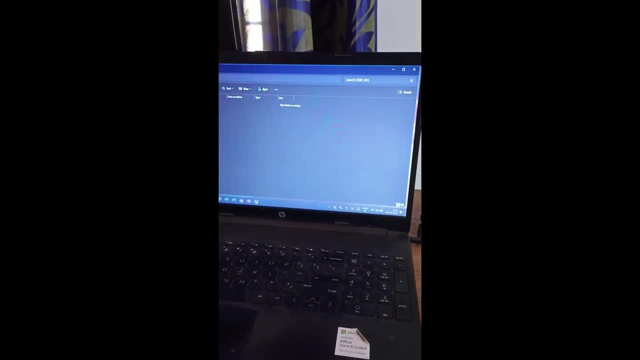 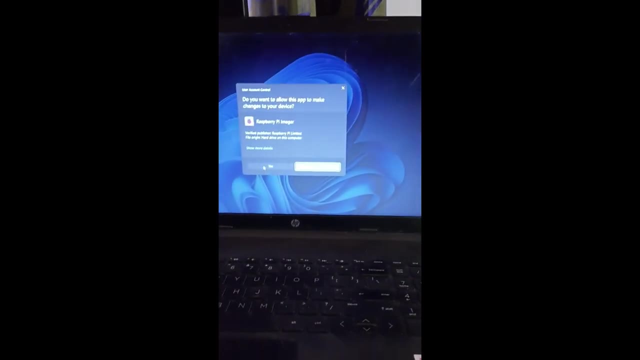 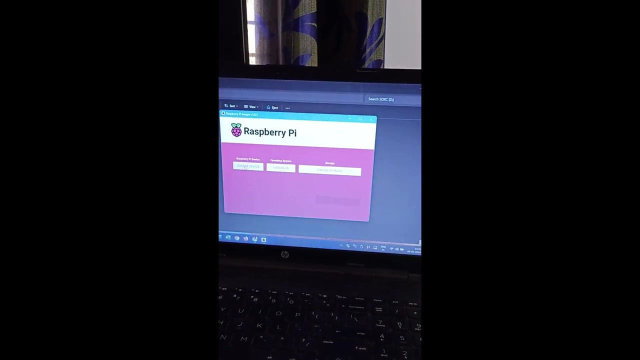 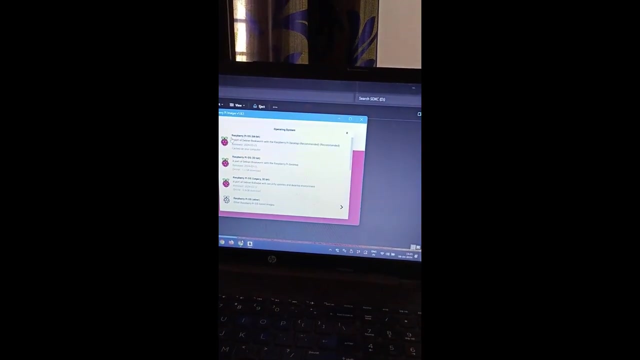 fully empty so I have to install the operating system inside this. so I will open raspberry pi imager. click on the yes button and you can see this small window that comes say choose device. I will choose raspberry pi 4 because that is the raspberry pi I have. choose operating system: I will choose this one. 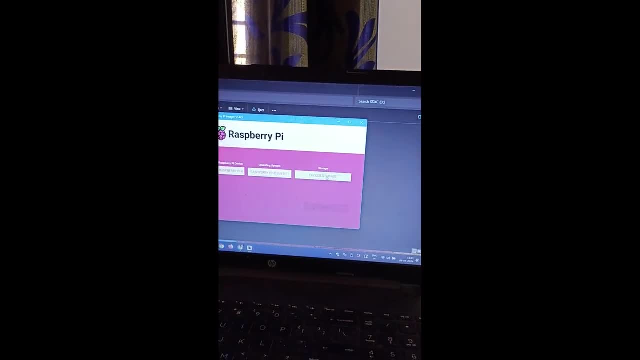 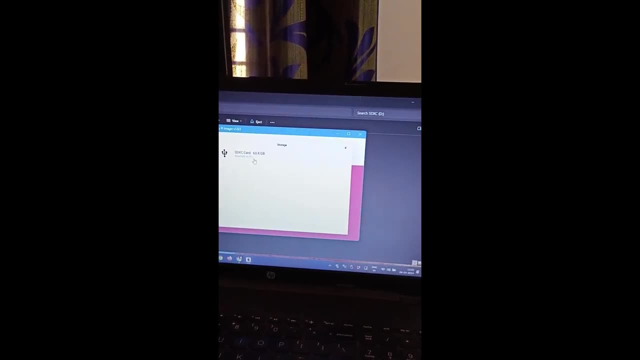 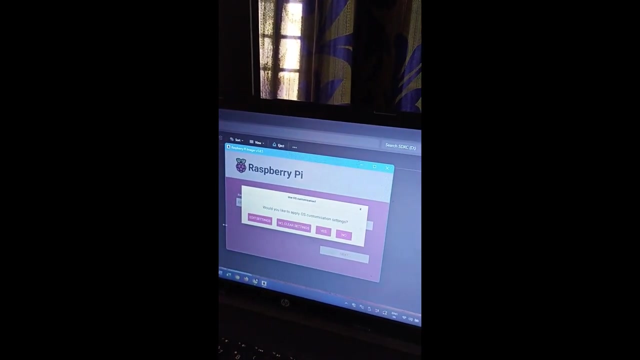 raspberry pi OS 64 bits and storage. as you can see, this is the SDXC card that is of 64 GB. it is mounted as D Drive. I will choose this one. click on the next button. it asked me: would you like to apply OS customization settings? I will. 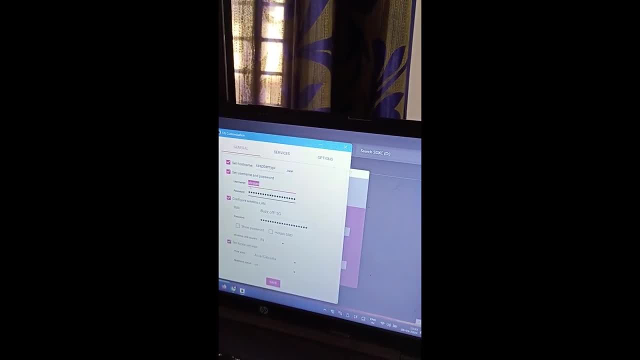 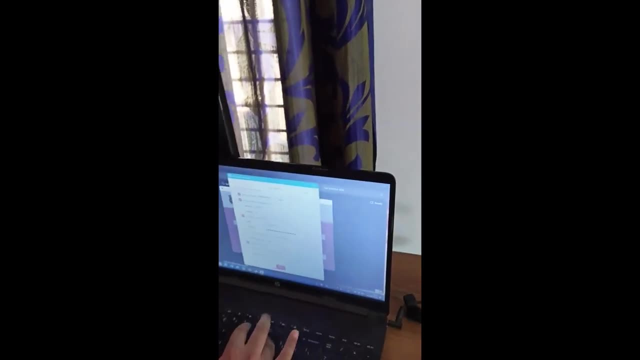 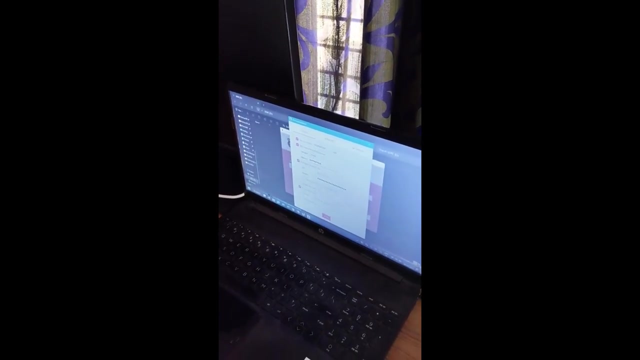 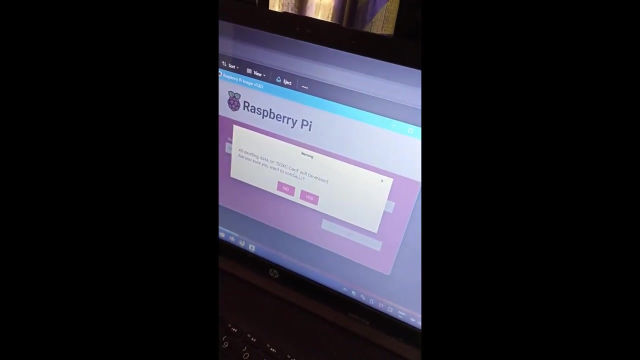 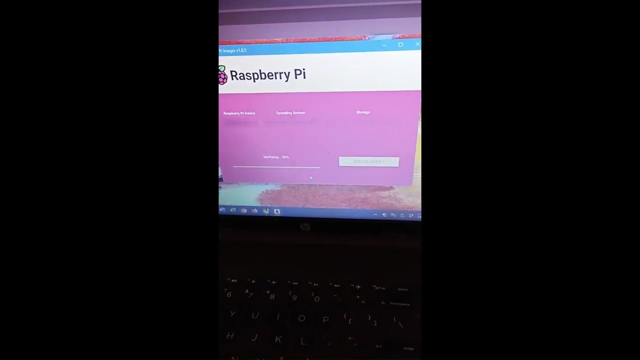 say, edit settings. here you can see what all I have made. you can change the password and use the password. you can change the password and use the password name and click on save and click on the yes button. all existing data on SDXC card will be erased. yes, it will format the SD card as you can see it is. 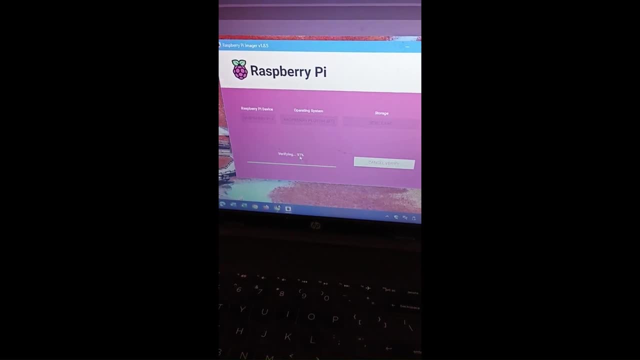 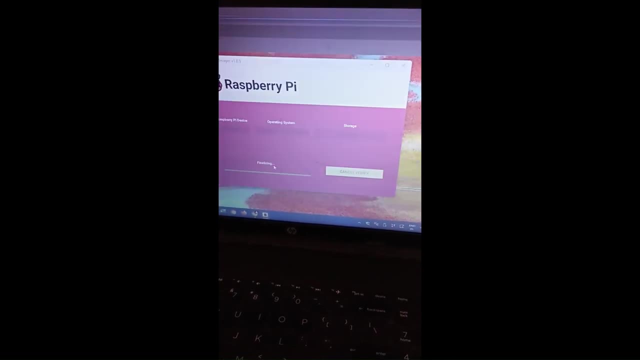 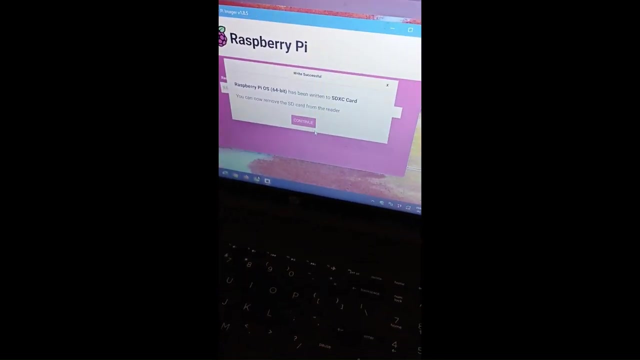 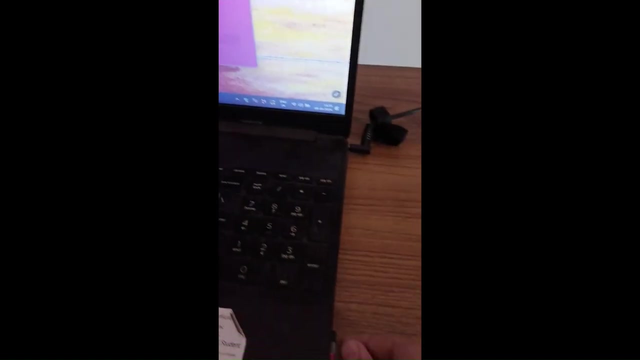 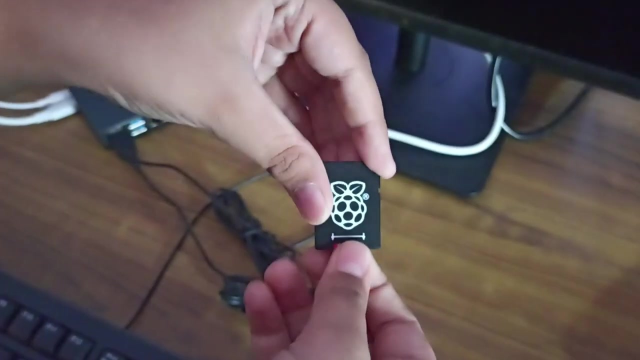 verifying it is almost done and yes, it is finished and this folder opened. you can see there are many files in it. you can see it is showing. you can now remove the SD card from the reader. click on the continue button and remove the SD card and remove the micro SD card. 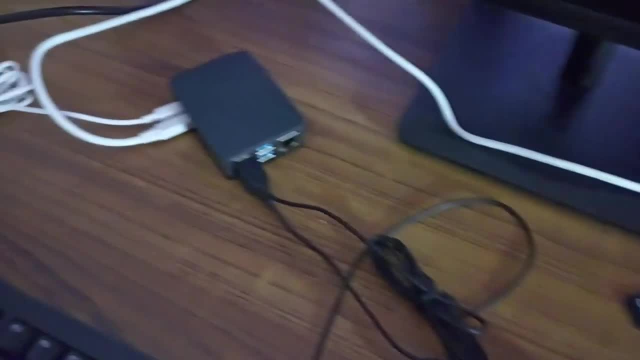 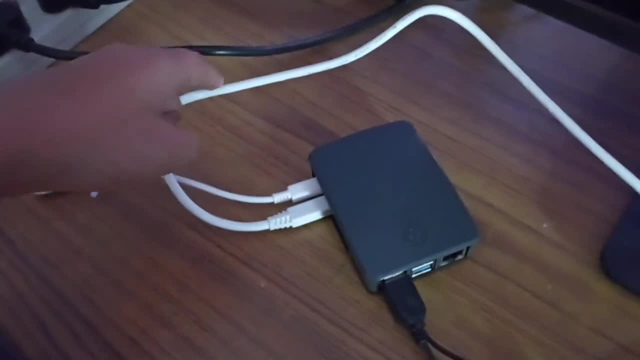 I have connected the adapter to the board. I have connected the adapter to the board. I kept the board inside the case the. this: I kept the board inside the case the this: I kept the board inside the case the. this is the micro HDMI cable I have connected. 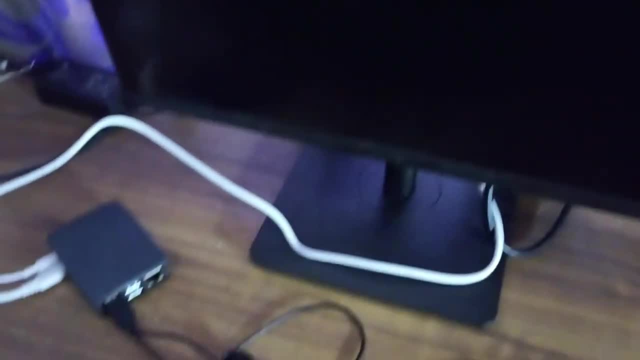 is the micro HDMI cable I have connected is the micro HDMI cable. I have connected to our monitor and I have connected the to our monitor and I have connected the to our monitor and I have connected the keyboard, the keyboard and the mouse keyboard, the keyboard and the mouse. 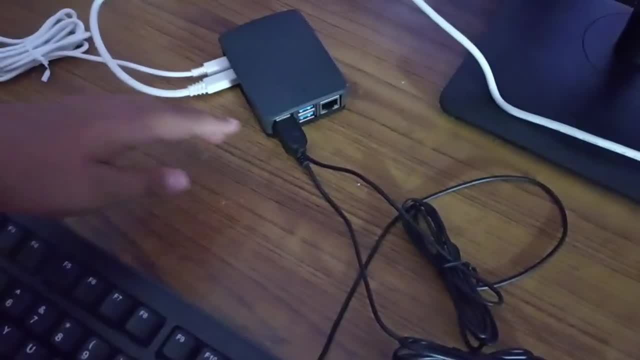 keyboard: the keyboard and the mouse. remember that you can use a Bluetooth. remember that you can use a Bluetooth. remember that you can use a Bluetooth mouse. after the setup: before the setup: we mouse. after the setup: before the setup: we mouse. after the setup. before the setup: we have to use a normal wired mouse now. 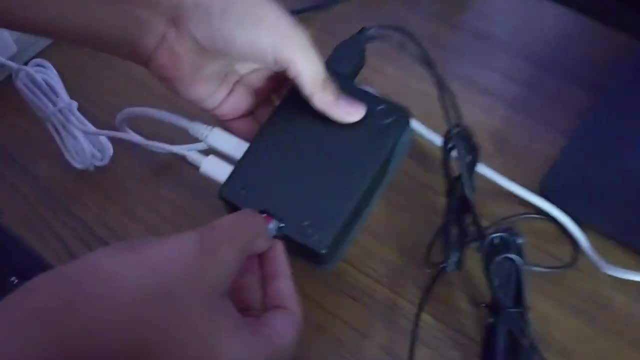 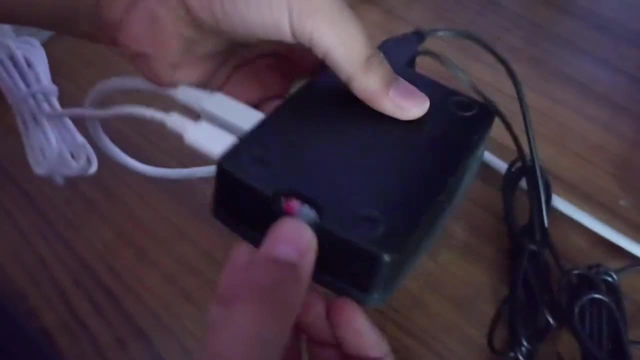 have to use a normal wired mouse now. have to use a normal wired mouse now. we will connect the micro SD card as you. we will connect the micro SD card as you. we will connect the micro SD card. as you can see, it is connected. next thing we 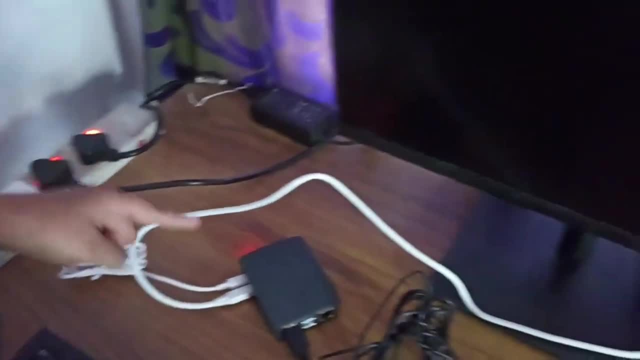 can see it is connected. next thing we can see it is connected. next thing we have to do is turn on, as you can see. it have to do is turn on, as you can see. it have to do is turn on, as you can see it is turned on. then we will turn on the.